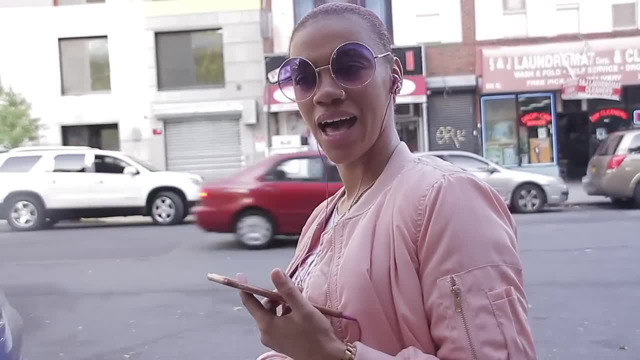 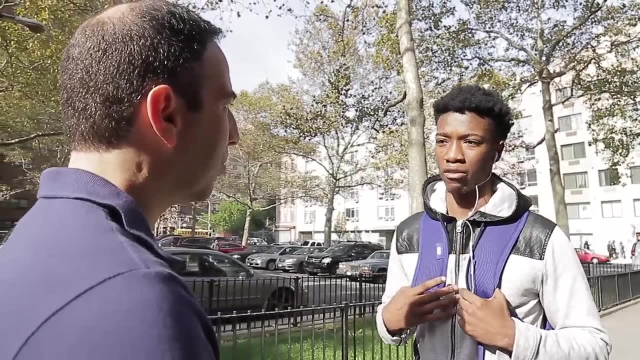 Why would they think we don't have ID? Ha, That's a lie. Why would they say that? Do you have ID? Yes, Because I have my ID and my friends have their ID, so we know what we need to carry around. 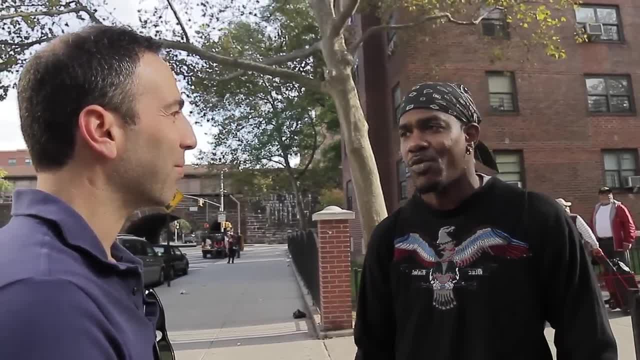 Everybody that I know have ID Like. that's one of the reasons, That's one of the things you need to walk around with New York with an ID. Do you know any black adult who does not have ID? No, I don't. 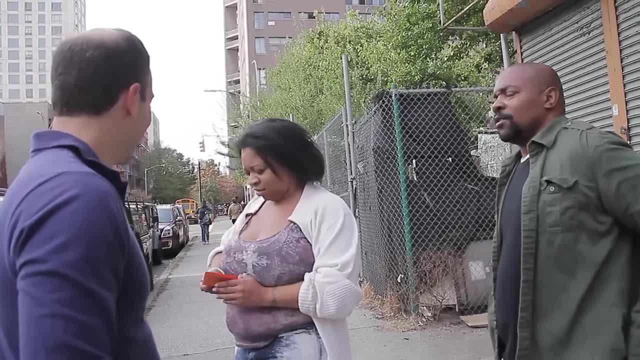 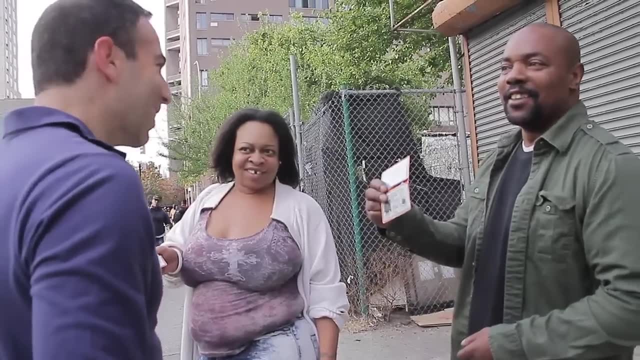 Is it a weird thing to even say that? Yes, it is. What is this? some type of trick candy camera or something like that? I know right, That's the only thing I brought with me. Those are legit IDs. I heard a lot also that black people can't figure out how to get to the DMV. 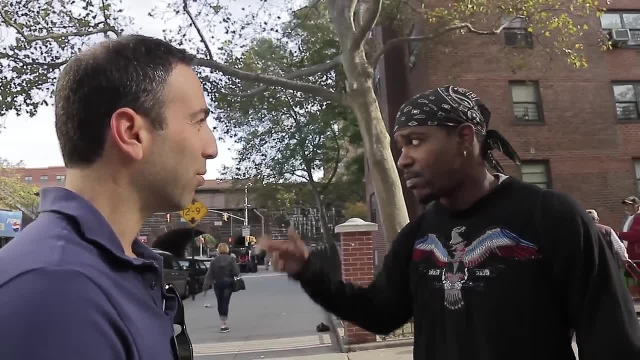 Really, What's that saying to you? I know it's that It's on 25th Street. Do you know where the ID, the DMV, is? right here? It's on 125th Street. It's on 125th Street and 3rd Avenue, I believe. 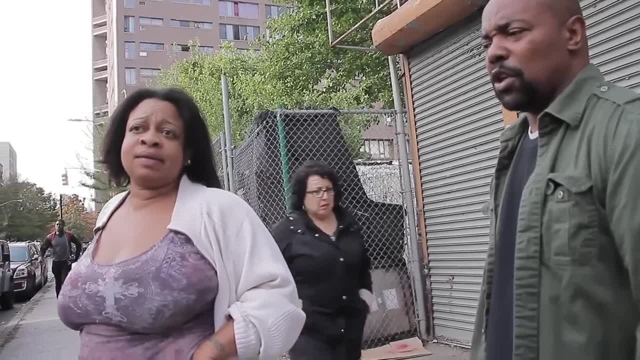 You know how to get there? Yeah, Do you have a problem getting there, if you have to get there? No, I know these sound like silly questions. You know how to get to the DMV? Of course You know where it is. 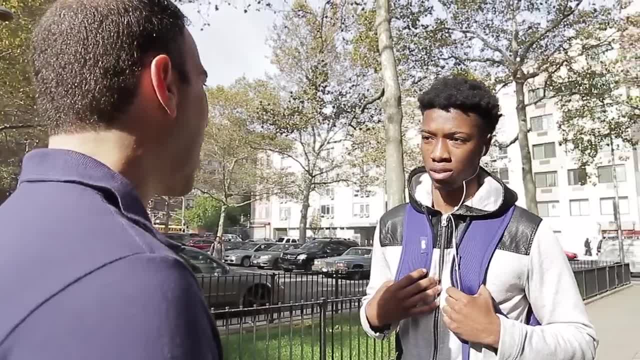 Yes, You can get there. Uh-huh, No problem, No problem, Just checking, Okay. And I also heard a lot that black people, especially poor black people, have no access to the Internet, can't figure out how to use the Internet. 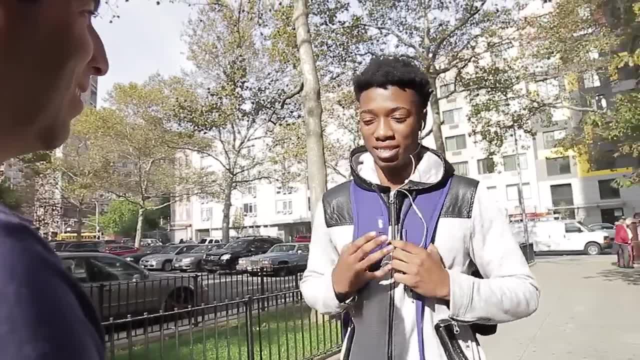 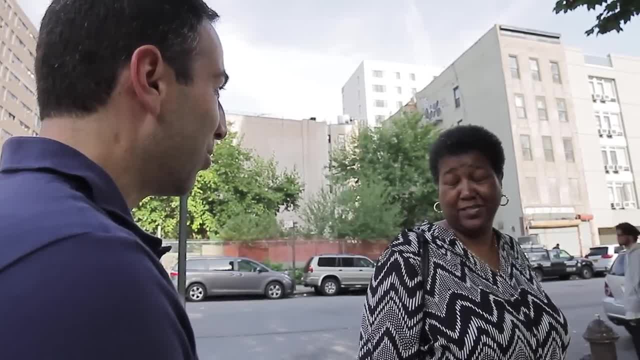 You know how to use it properly, right, Exactly. I do it at work, So of course I know how to use it. My kids know how to use it. They all have iPads, iPods, whatever Your phone has data. 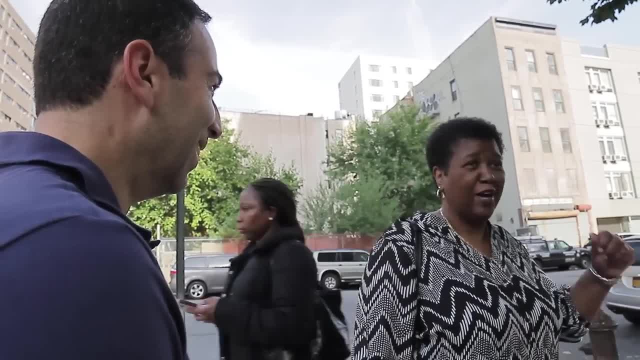 Uh-huh, You can actually Unlimited- Unlimited data. Uh-huh, I use my phone as a hotspot. What does that say to you? for the people who have this perception of black people, They're pretty much ignorant. That's what my thought process is. 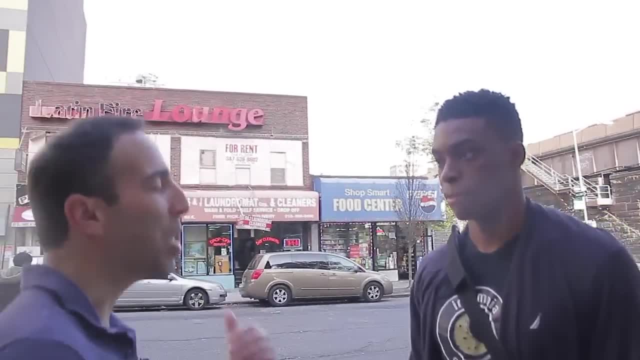 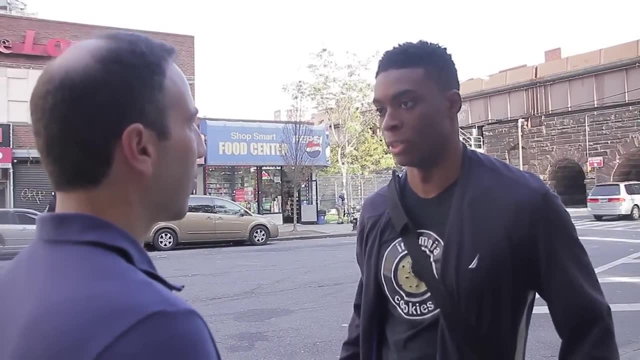 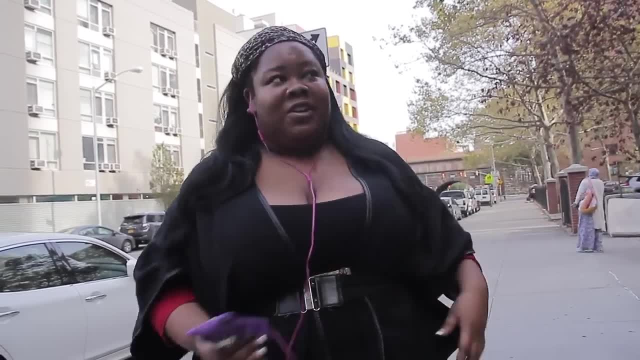 Very, very ignorant, Ignorant, Very, very ignorant. Does it sound racist for somebody to say that? I think it is a little racist, because you know you're putting people in a category and you have no idea what you're talking about. 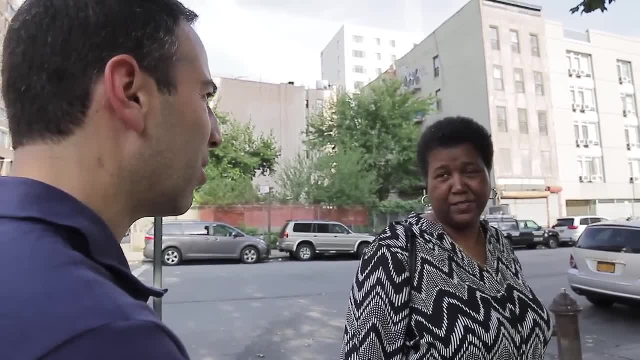 Maybe a little bit of racist in it but, like I said, I think it's more stupidity and ignorance. You're judging somebody like, but you're judging them for they're black, saying that they don't got it. What people are they talking to? 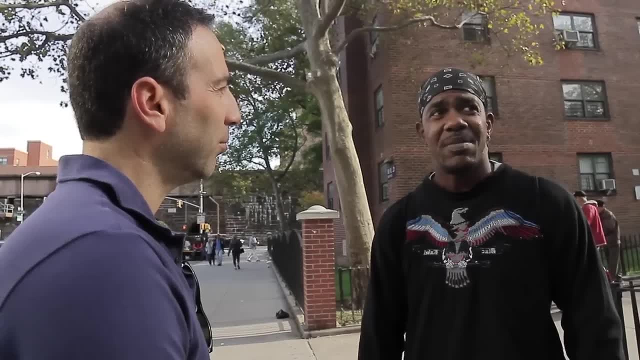 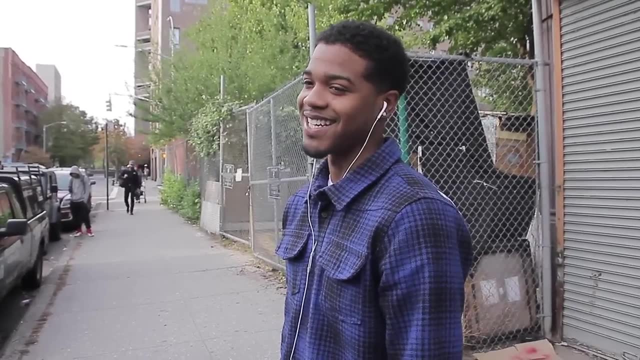 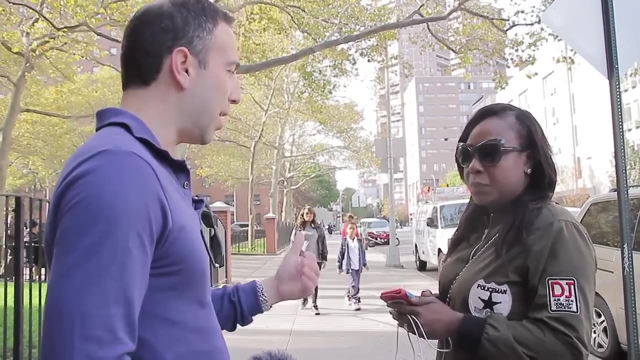 What are? Who are these people talking to? Do you have a problem that if you go to a black person's house, they don't know what they're talking about? No, No, No, No, No, No, No. If you go to vote and they say, can we please see your ID to make sure you are who you say? 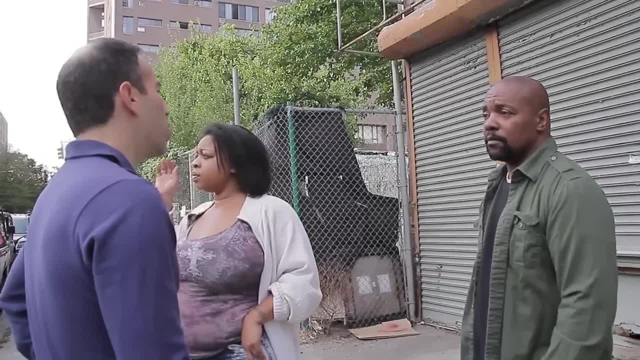 you are. I love showing my ID. You have no problem with that. Nope, Would you have a problem if, when you go to vote, if they say: can we please see your ID to make sure you are who you say you are, do you have an issue with that? 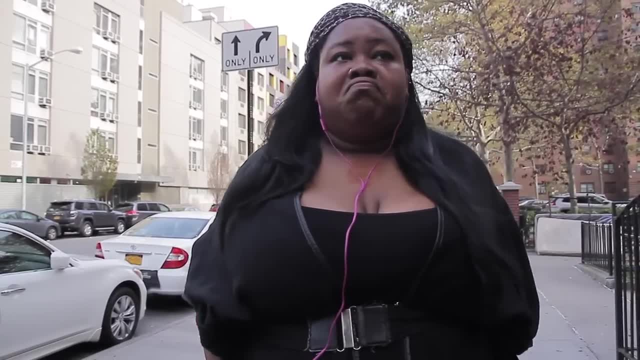 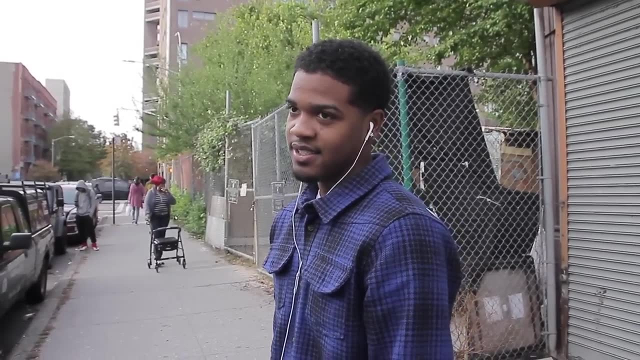 No, Would you have a problem if there was a rule where you had to show your ID in order to vote? I don't think so. No, Would you have an issue if there was a rule saying you gotta show your ID before you vote? 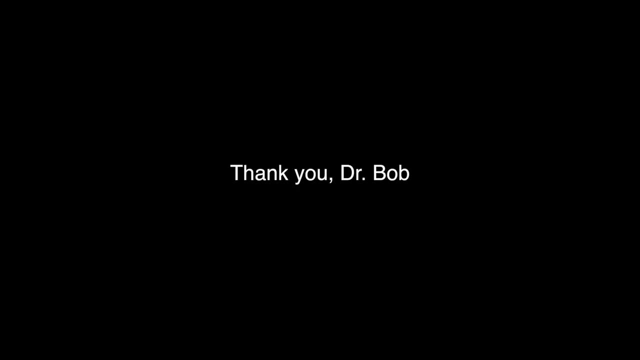 Nah, Are you cool with that? Yeah, Yeah, Yeah, Yeah, Thank you.